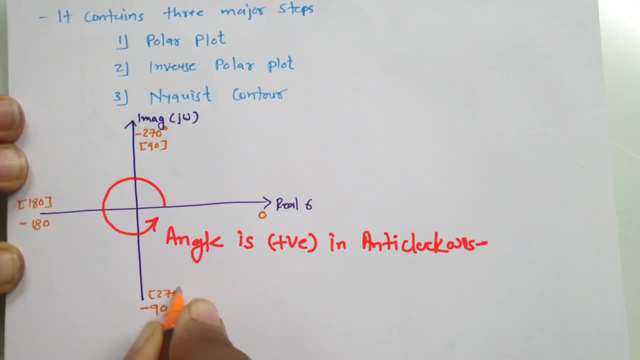 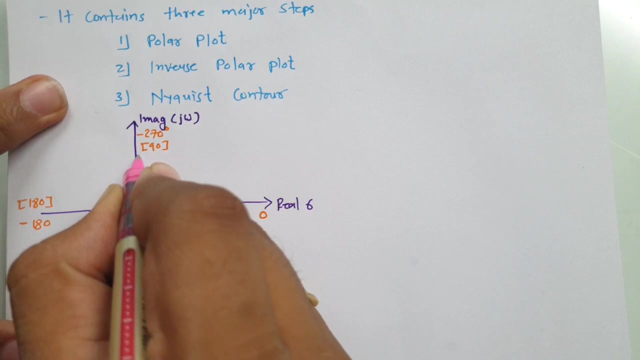 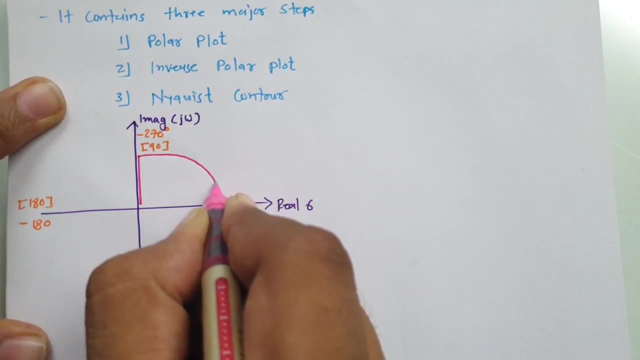 Right. That is how angle is Right. That is how angles are there. Now let me explain you all the steps which is required to understand Nyquist contour. So you might have seen this type of Nyquist contour in textbook, Right? So I'll explain you this entire contour step by step. 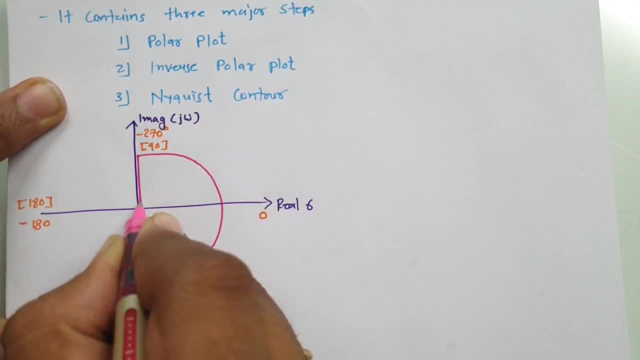 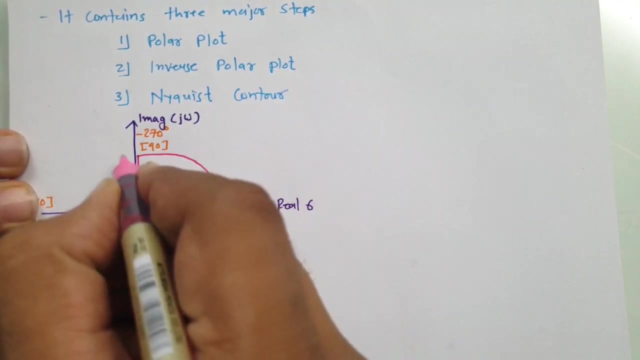 Right. This is how you might have seen one contour and that is what Nyquist contour. Right And based on this Nyquist contour only, we are delivered to plot Nyquist plot. Now let me explain. here, see, angle is 90 degree and here angle is minus 90 degree. 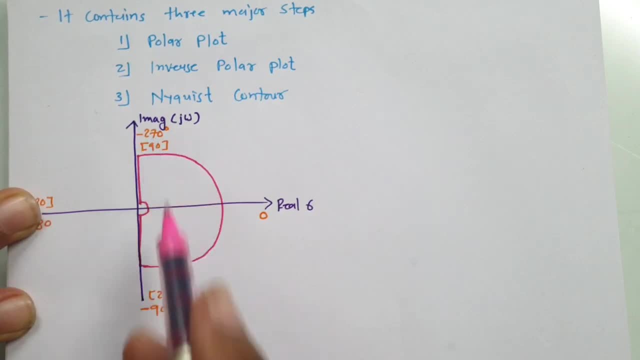 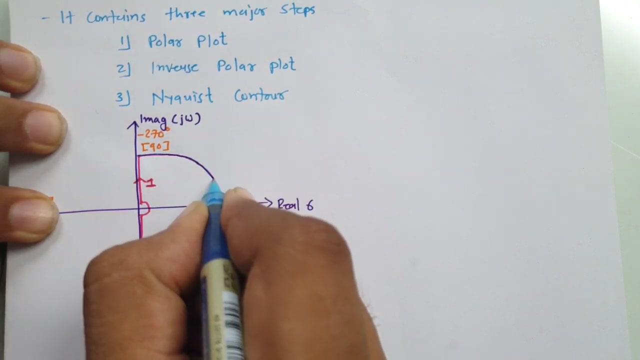 Right, And even you can say: this is minus 270 and here plus 270. And when we talk about this Nyquist contour, then this Nyquist contour that is bisected in four different part. This is part one. Then if I say this is my second part, then this is my part two. 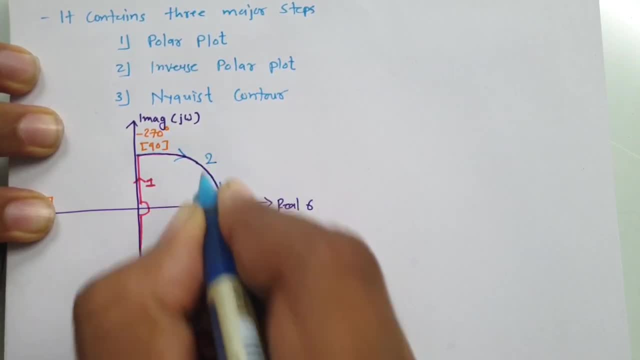 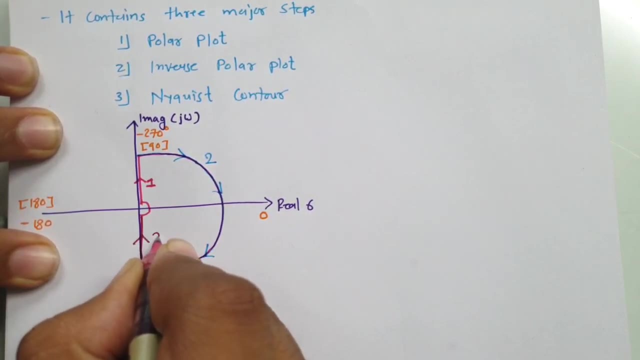 So that is happening like this, You see, And as if I say this is my part three, then see that is happening like this: This is part three. And See This Small Circle. That is possible, as if poles are over here. 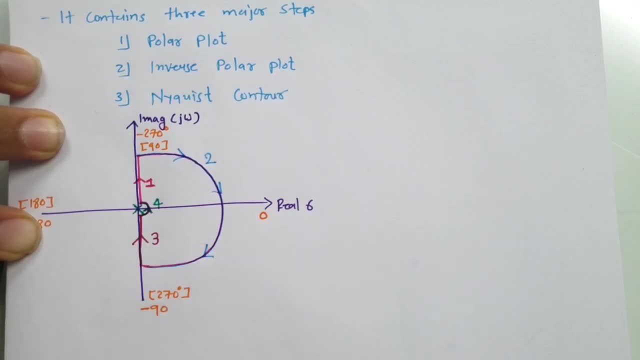 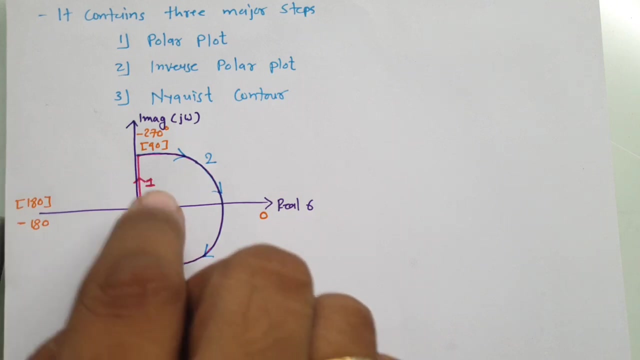 Right. So this is part four. Right Now Let me explain you how to calculate all these four parts step by step, and that is what resultant Nyquist plot. So how to plot all these four parts- part one, part two, part three and part four- one by one. 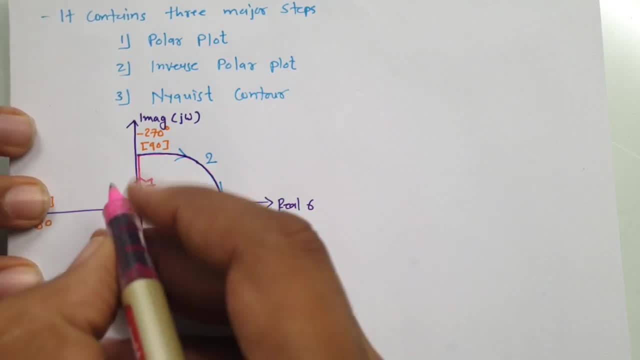 I'll explain you that. So, when we talk about this part one, I'll explain you that. So, when we talk about this part one, So here I'll tell you, With this part one, You see, So in this part one, 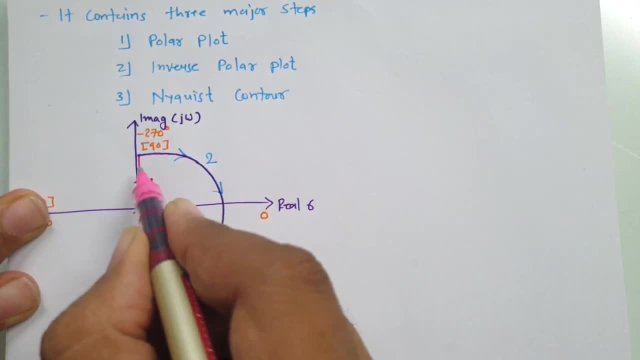 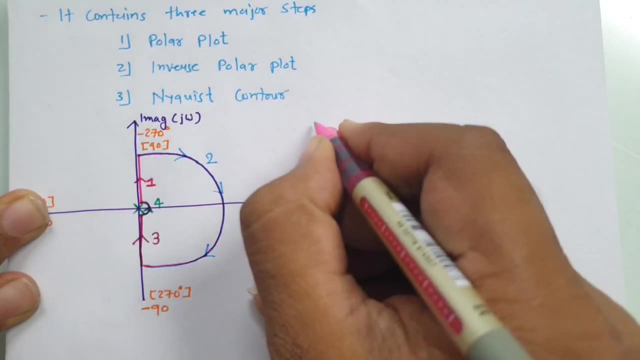 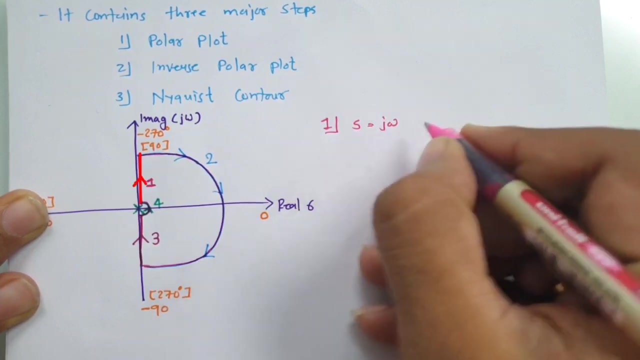 We are delivered to a place As is equals to u j omega in the system, And that is the plot of Nyquist plot. So you see, for this part one, We are delivered to place As is equals to J omega, and that is Polar plot. 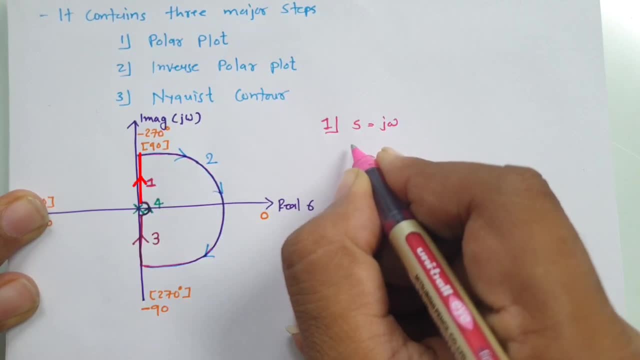 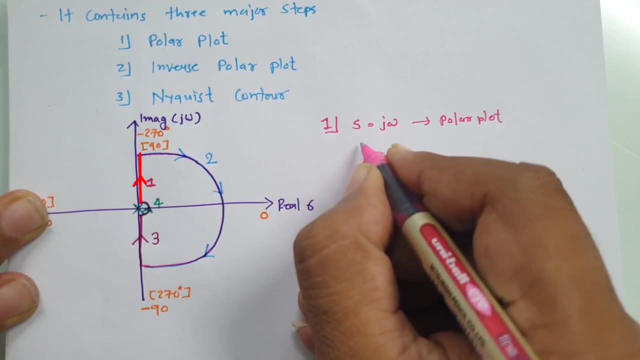 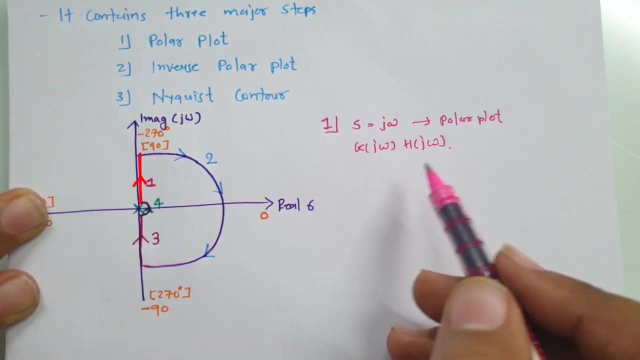 Of system JFS H s Right. So this is polar plot where you will be plotting g of j omega, h of j omega. So how to plot polar plot, that I have already explained you in my section of polar plot. You just go through that. definitely you will understand how to plot polar plot. 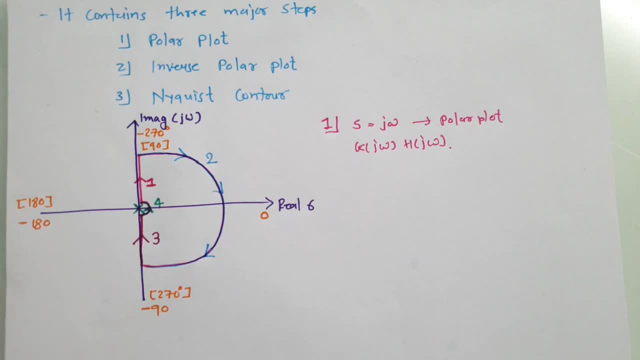 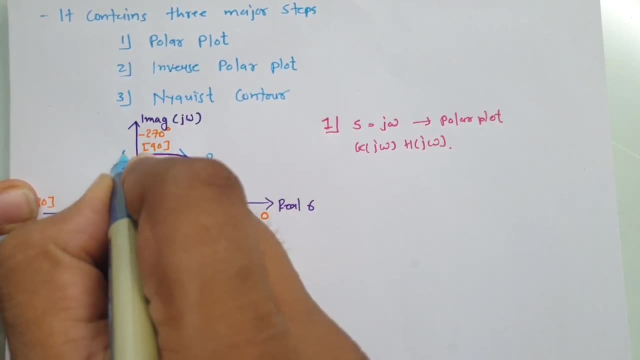 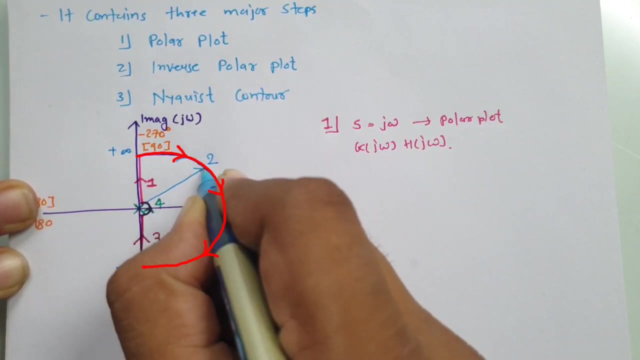 Now, in second section, you see here big contour is there and this contour that varies from plus infinite to minus infinite and if you observe this is the radius, then that radius is tendings to infinite right. So this contour that is r into e, to the power, j, theta, where theta varies. 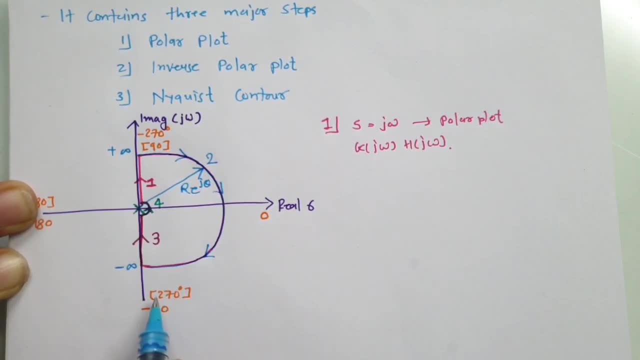 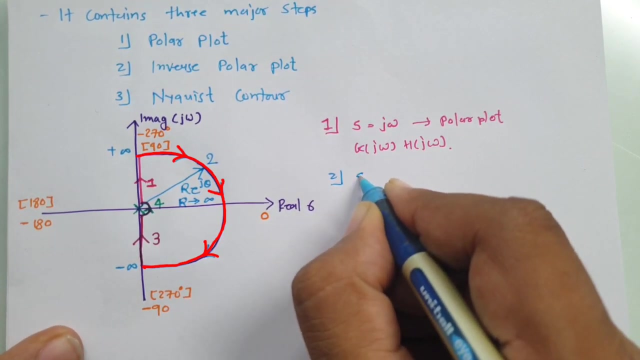 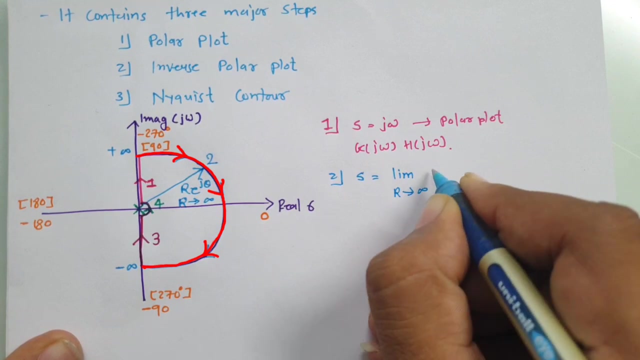 from 90. To minus 90 right and r is going towards infinite. So this is my second part of this Nyquist contour and in this Nyquist contour we are delivered to place s, that is, having limit. r tends to infinite, r into e to the power. 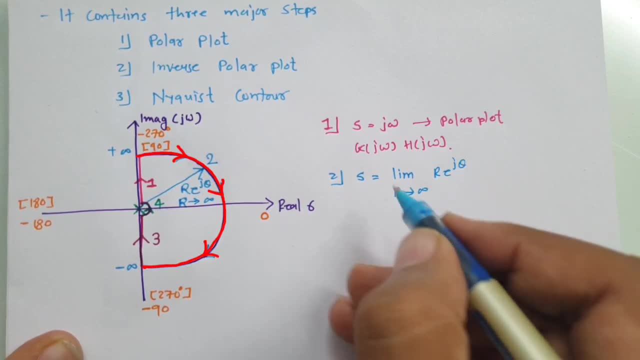 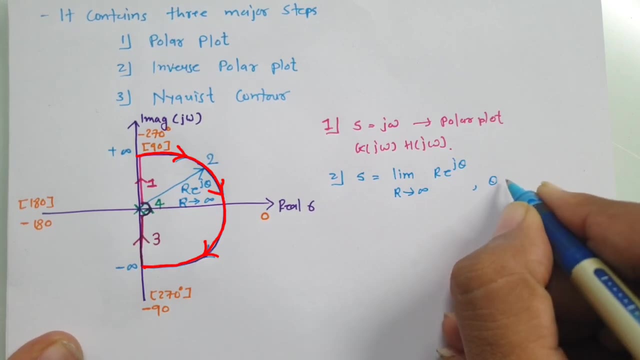 j theta. So this is what you will be replacing by s In given systems transfer function and in this theta that will varies from 90 to minus 90. you see, it varies from 90 to minus 90.. So this is what our second part of this Nyquist plot and see, once you place this all we will. 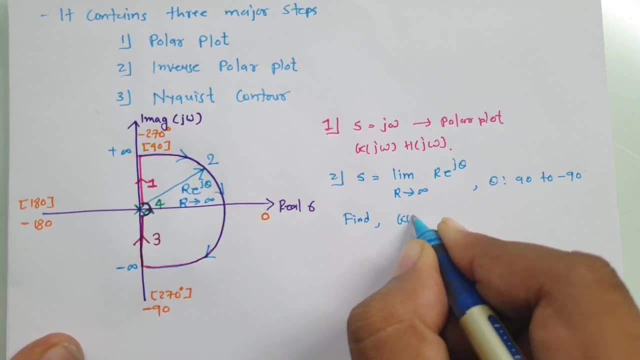 be doing is we will be finding g, s, h, s, And that is the number of points that we are going to be placing. So this is what we will be finding by limit r tends to infinite. g of capital R e to the power j theta. h of capital R e to the power j theta. 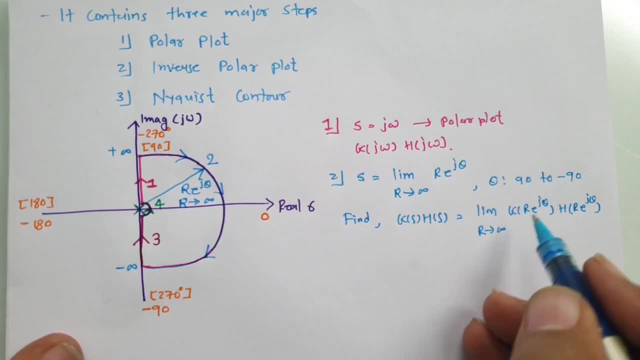 So we will replace s by r into e to the power j theta and we will try to identify magnitude and phase variation. So in example I will explain you how to calculate those things. It is very easy Right now. you just understand these steps. 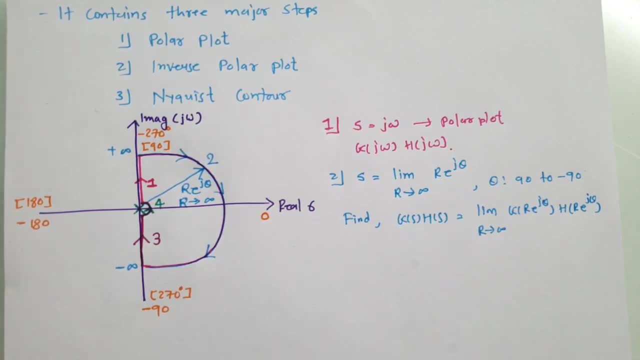 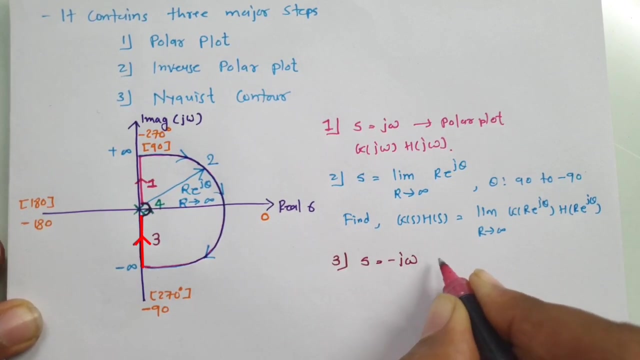 Right now, in third step, if you observe. So this is the line which we are delivered to cover. So in this third step, you will be observing, we are placing s is equals to minus j omega right. So in third line step, you will be placing s is equals to minus j omega right. 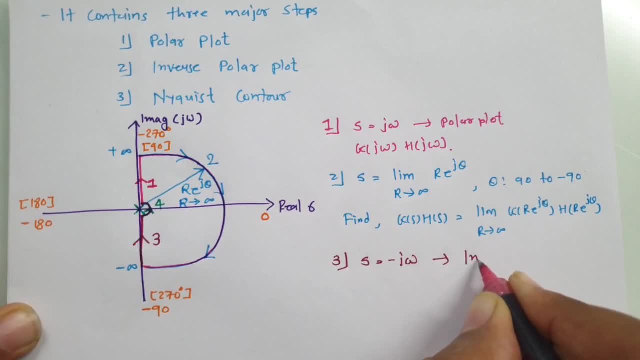 And that is what inverse of polar plot. That is what Inverse polar plot And that is what you will have to plot it with respect to real axis. So whatever polar plot that we have plotted for this line one, So with respect to real, we need to have image of it. 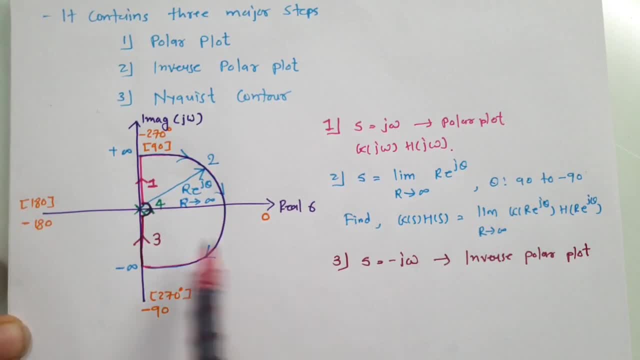 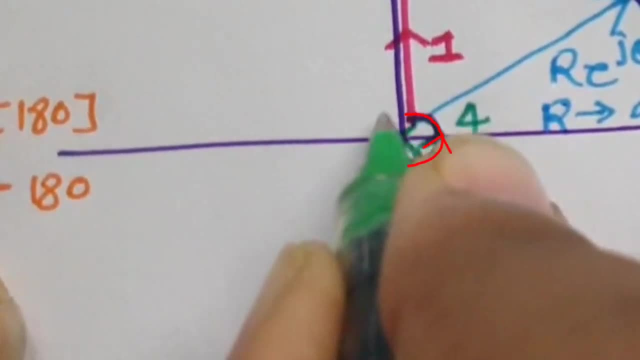 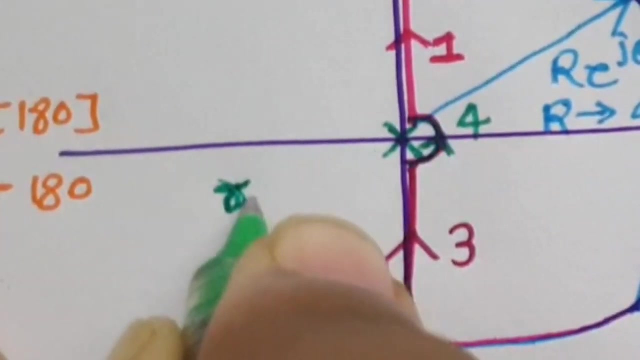 So that is inverse polar plot, Right? So that is our third section. And if you observe this small circle, Right? So in this small circle You will be having radius, small r, into e to the power j, theta, Where now you see, theta varies from minus 90 to plus 90.. 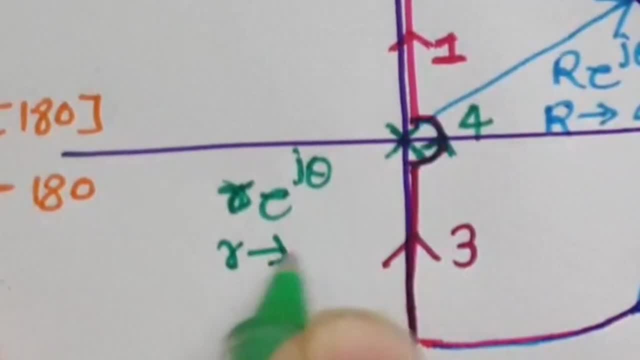 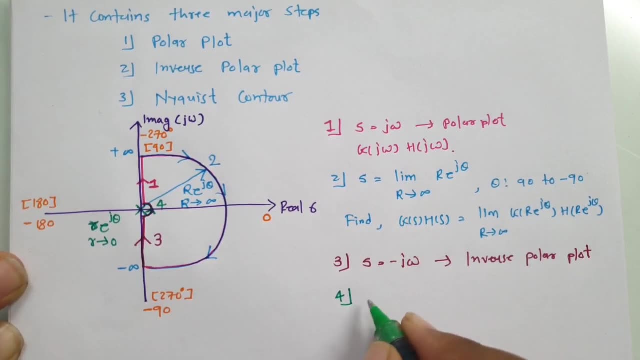 And this radius is tending towards 0. Means radius is very small for this Right. So in fourth part all we will be doing is we will place s is equals to limit this radius r tending to 0. So r e to the power j theta, where this theta will vary from minus 90 to plus 90 right. 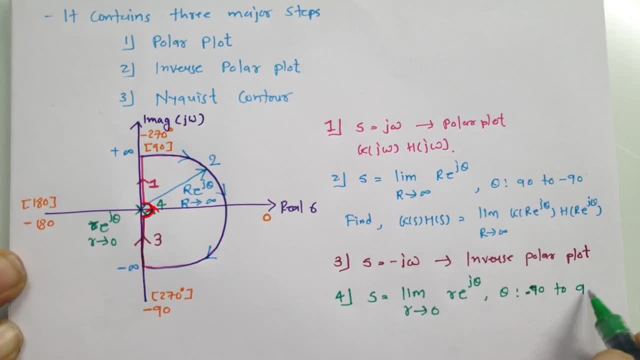 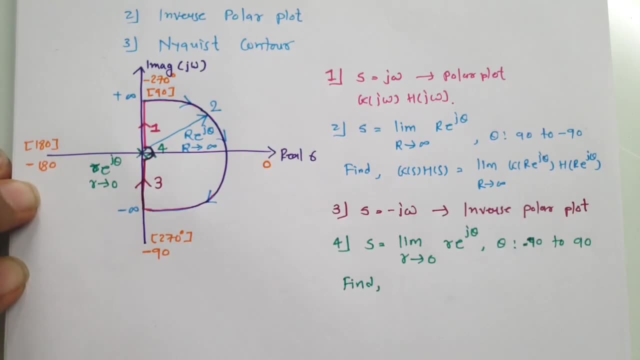 So minus 90 to plus 90, variation of angle will happen And we will be finding value of g, s, h, s, where limit small r tends to 0. g of small r is equal to 0. Right So g of small r e to the power j theta, h of small r e to the power j theta. that will be. 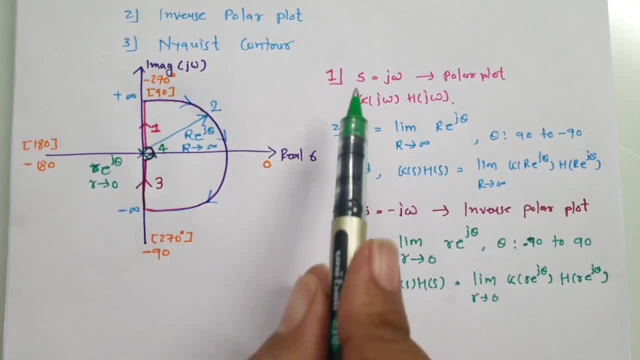 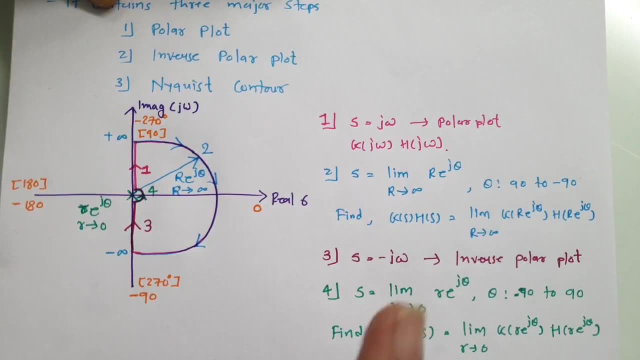 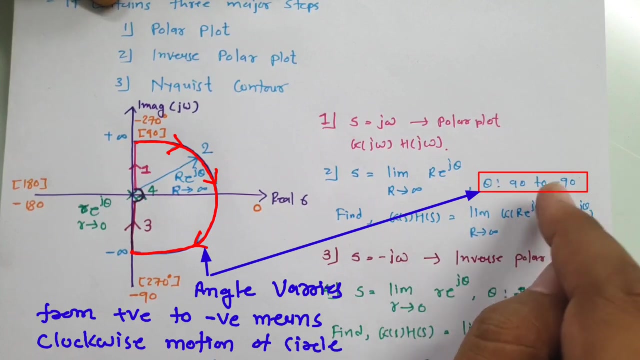 the calculation that we will be doing, And once you have all these four steps covered, we can have a complete Nyquist plot Right Here. one more thing that one should focus about, As if angle varies from positive to negative, you see, from 90 to minus, 90 variation of Nyquist.